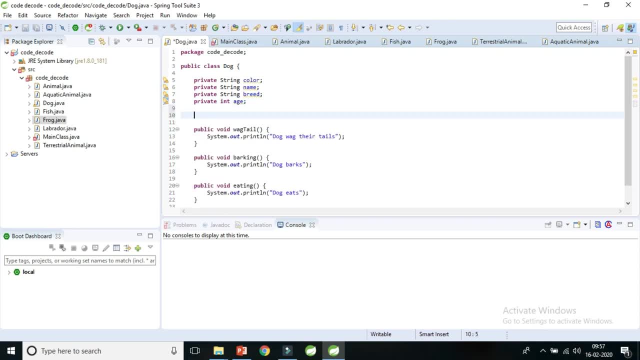 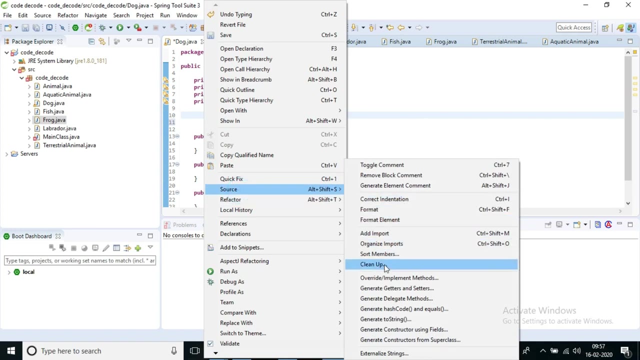 So these were three methods, which was already present. These were the methods of a doc class. Now I want to use these: color name, breed and age of the doc class. So what I will do is I will right click here, I will go to Source, I will go to Generate and Geters and Setters. 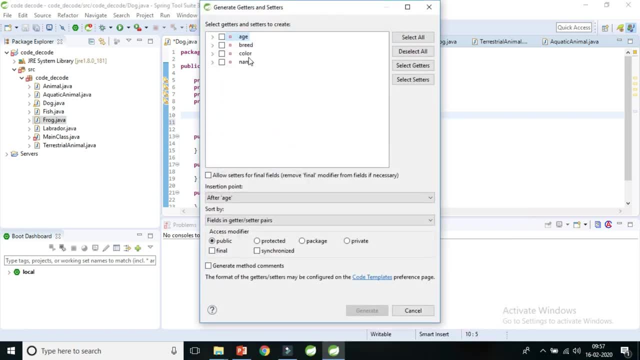 So do you see this method: Generate, Getters and Setters. So it gives me a check box. If I want to click all of them, it will create the getters and setters for all of them. So as of now, I will select both, all of them. So I will do Generate. So what it does it. 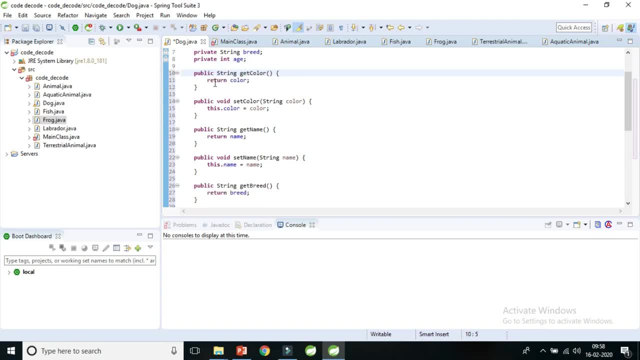 does nothing but creates public getters and setters there. As you can see, that is how getters and setters for us right see? all these are public getters and setters for us. so this is how i have implemented encapsulation. but the main part here arises is that: how does 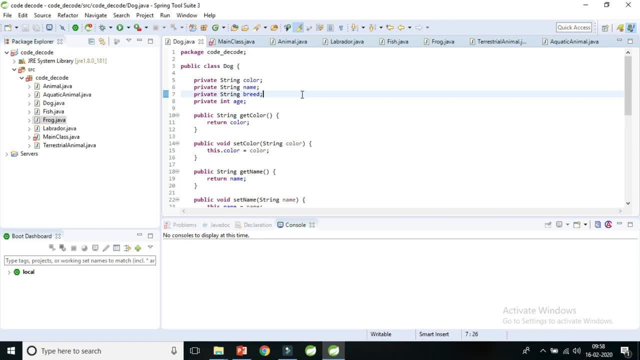 that benefits us. so, because even the work was even being done earlier, so how does it benefits now? so the very first and important part of this was that if we achieve data hiding, so how do we actually achieve data hiding? so this was my main class right, so in this main class, 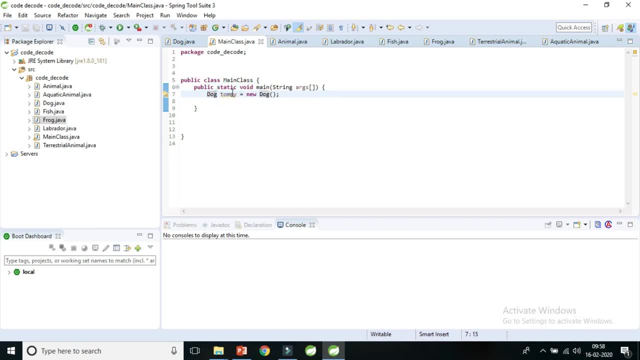 i have created my object tommy of type doc, right, so this was my class, which has private variables and public methods. so i've created an object of this tommy. now, if this is another class, this is called as main class, so this is an outside class. so if i try, tommy dot and i'll print. 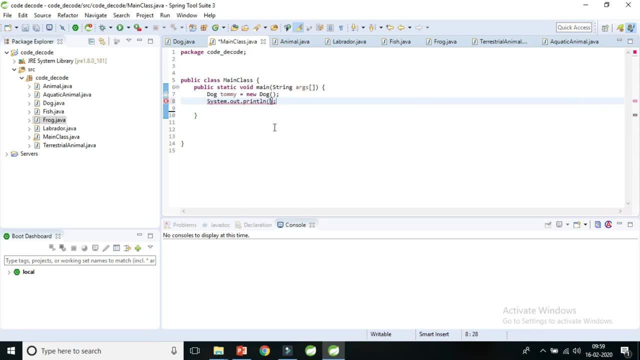 it. so let me just write it in: see so itself and I'll say Tommy dot, age. so it's giving me an option of gate age or set age, but it is not giving me an access directly to the age object or variable. so what it says change. 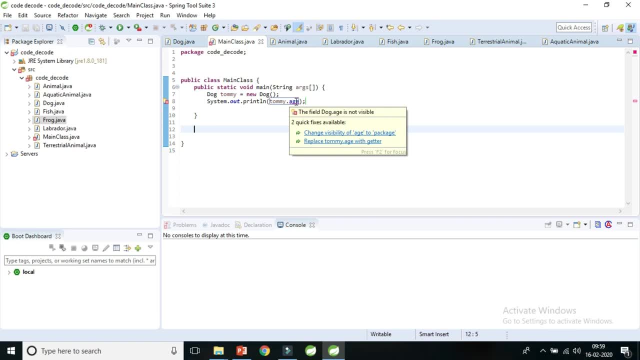 visibility to package, because it is currently private and all the effort you can replace Tommy don't get with the getter of this particular method. so if I replace it with it, so it gives me a getter of it getter option. but as of now I I'm trying that this particular object should directly access my age variable. 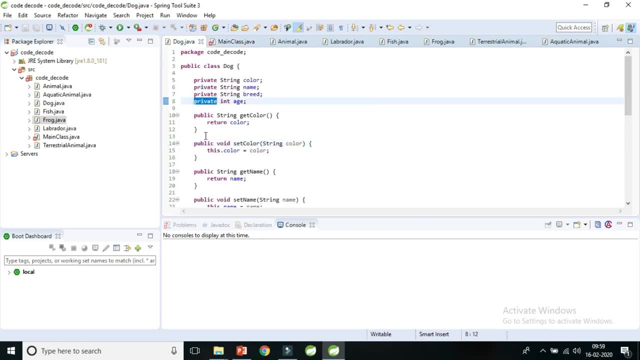 but it says me no. so this is the beauty of encapsulation. so if I deleted, I don't make it private. what happens, it's very good. it doesn't give me any compilation error, it can- even I can easily access age with just creating an object of it. 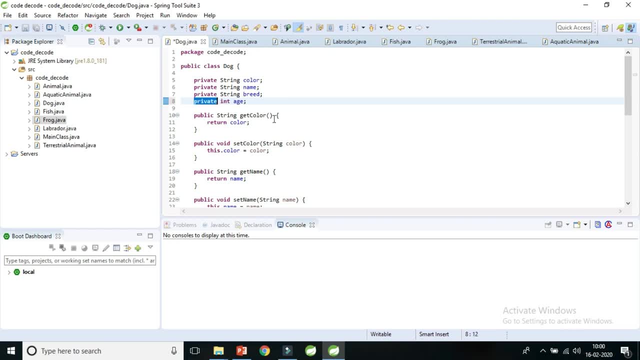 rather than creating the method, creating it private. so this is a beauty of encapsulation. second advantages of covered earlier in the theoretical view is that by creating the getters and setters you can make a class read only or write only. so currently what you can see is you have getters and setters, both. so if I create only setters and not the 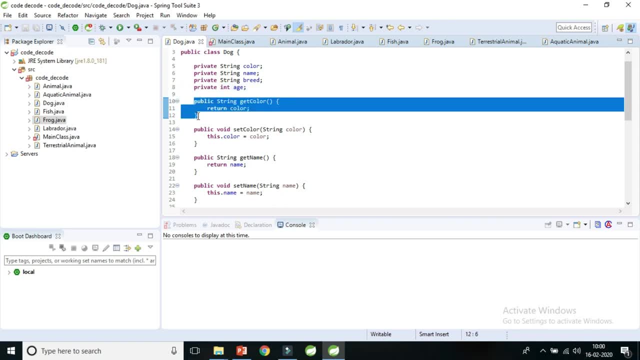 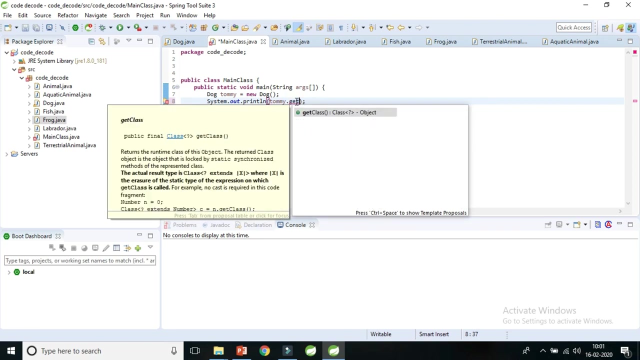 getters. what happened? so I'll remove this for you. okay, I'll remove all the getters. fine, I've removed all the four getters for you. I only have setters now. what will happen now? see dot age. I cannot do for sure, dot get. now getters are removed. I'm not getting any option of, I'm only getting. 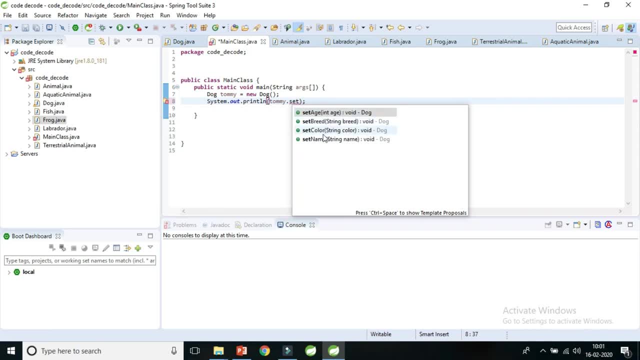 in the options of setter. so what options I'm hitting age, period, color and name. I'm only getting the options of set. so what options I'm getting age, breed, color and name. so I can only set my data. say, I set my age as 15, but can you see I cannot read. 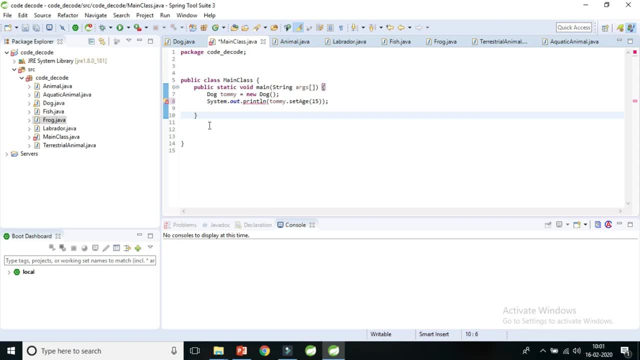 any on any such data. it says argument matching. sorry, I'm setting here. so this is. this should not be done here. you can do it in another way, as Tommy dot set age as 15 and I can save it. age is private. that is why it's giving compile. 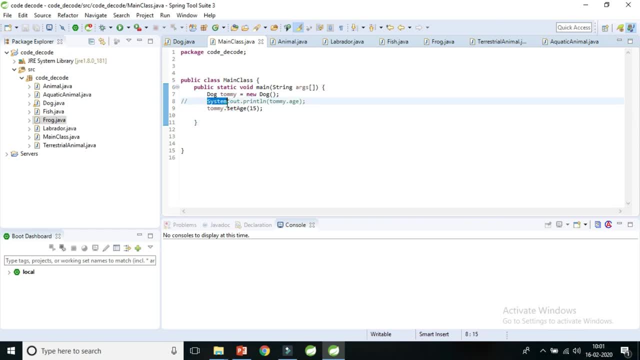 time error so I can save it here easily. so what I'm trying to do here, I'm going to set my age, but I cannot see it. I cannot do get age, why? or neither can I try with variable. so this is how: I cannot get any of these variables and 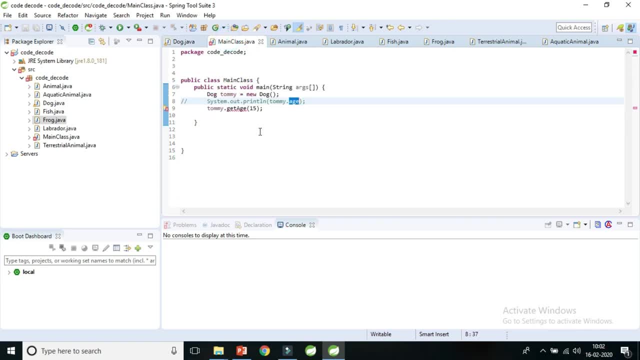 hence I cannot see any of the values being set here. I can only read it by, I can only set it, I can only write it. so this is right. only way of implementation of a class: by only using setters. what happens if I use only getters and not the setters? so I'll remove these setters for you now, if I 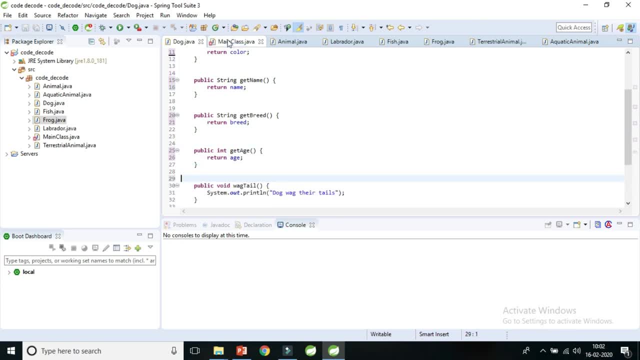 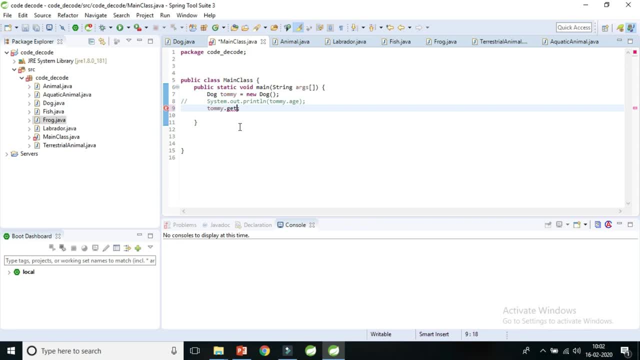 something onto your screen, you cannot set anything, and hence you can only get or you can only read, so this makes your class read only, and not at all writable or updatable. so this is another advantages of this. getters and setters, let's get back with everything, because actually both are important. we need read. 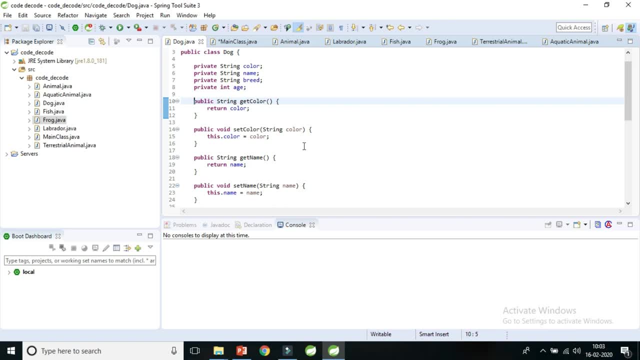 write and updatable class. another last advantage of encapsulation that you can see here is that you can control what data is being set here. so how can you do that? I have a setter here. right of age now if I say if age is greater than zero. so I've given. 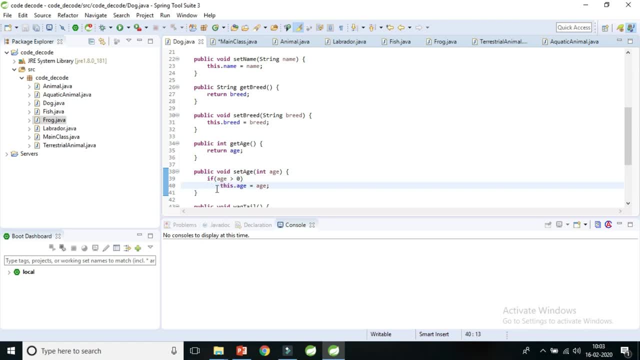 this condition only. if you are setting the age, then only set the age right. so I am going to set my age as fifteen and I'm going to print my age. syso and tommy dot get age. what I am going to get run is java application so you can see fifteen. what I've said I've 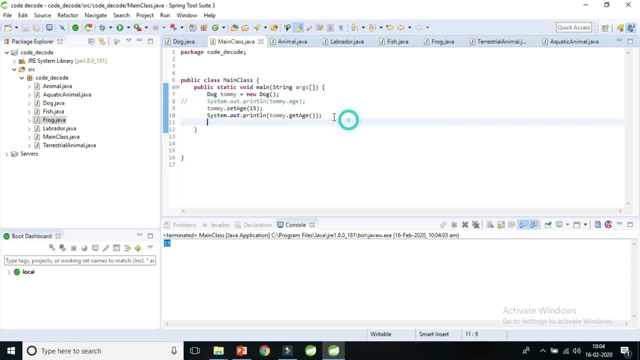 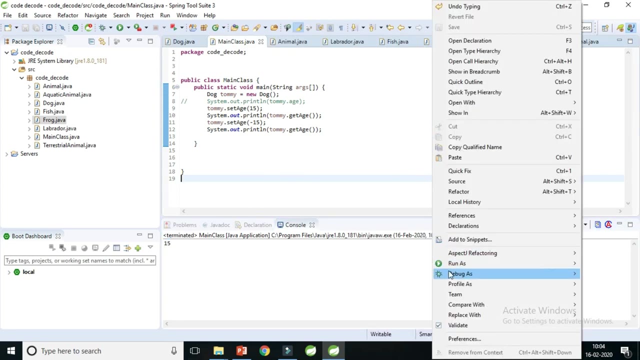 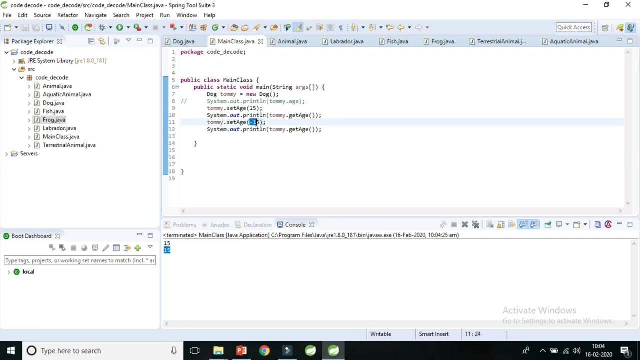 got, but nothing is going to be Read all at once. so atanniaptnet saves values here. so now, if i'm trying to set it and i'm going to print it, but not to 15 but minus 15, what will happen? it says 15, only it does not set as minus 15. why? because 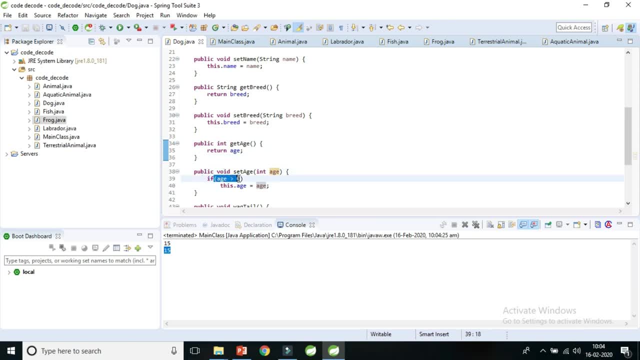 i have given in a particular condition, that only if age is greater than 15, then only set it, else don't set it. keep it as it is. so if i remove it from here, i'm not setting anything here. initially it was null, so if i try to run it i get zero. there is nothing i can do. 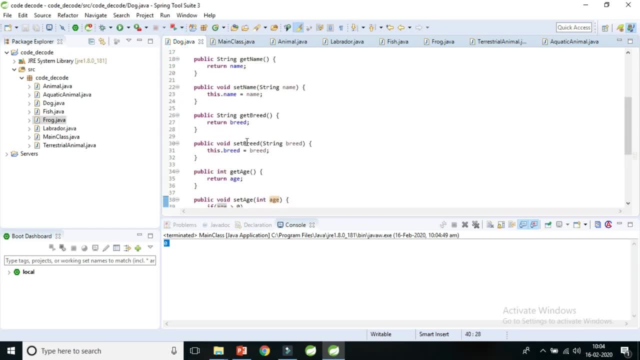 with the negative numbers here. why? because the default value for this int variable is zero. so the default value is: the value gets printed. it does not get printed with minus 15 or if. even if i say minus 5 and let's try to run it, even then also it will say me 0 because any negative number is not being. 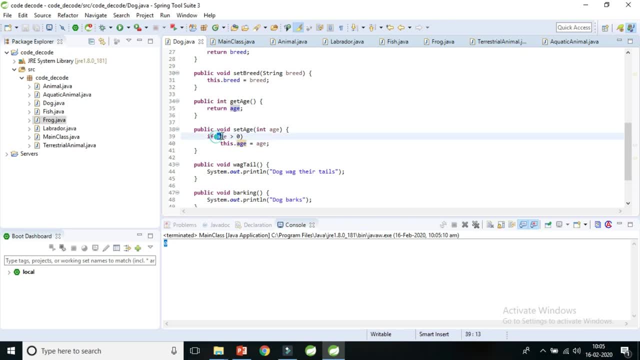 considered a particular variable which is satisfying this condition, h greater than 0, and hence it is not being saved. so this is very important. advantages of encapsulation: the first: i have seen that it is very easily generatable. these getters and setters are easily generatable by any ids. second advantage: that the getters and setters gives you data hiding the main class. 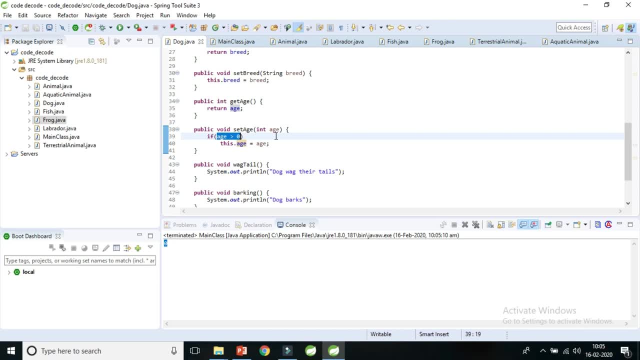 cannot access the dog class age variable when it is private or anything. you have to use the getters and setters to get or put the data into the class. the third advantage is that by providing getters or setters optionally, you can make the class read only or write only. 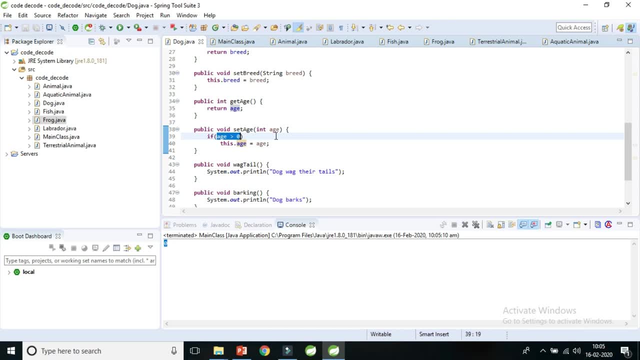 and the last one is that you can provide the control what data is being saved in your class as an object. if, if the age is not greater than 0, don't save it in this class. don't, don't corrupt the data. so this is how you can put your logic in these sectors. so that was all about the how. 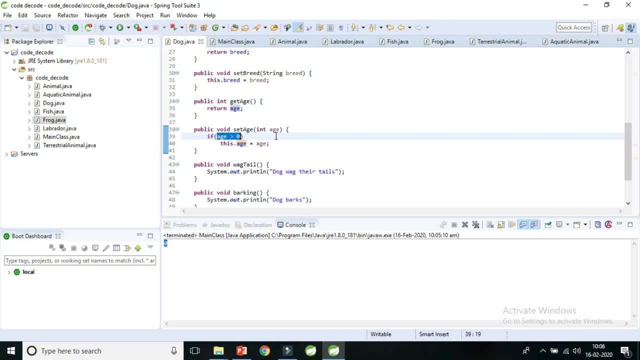 to implement the encapsulation, how to actually put your logics into it, how, what are the advantages of these encapsulations? i'll cover more such concepts, so please stay tuned, thank you.